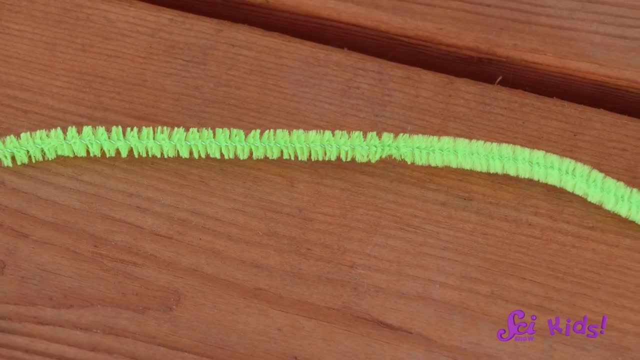 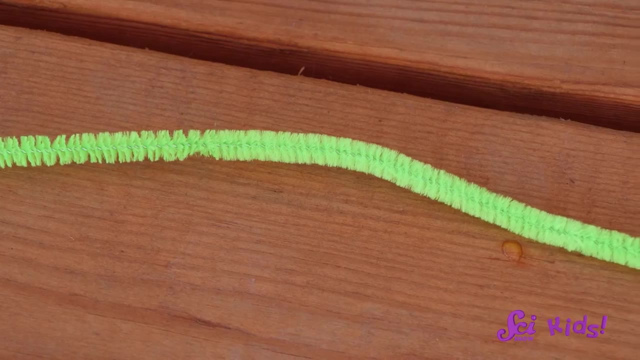 Now I have this chenille stick. It's kind of the same shape as the straw. Do you notice anything else about it? Squeaks, I agree, it's super fuzzy. I wonder what will happen if we put that in the soda instead. 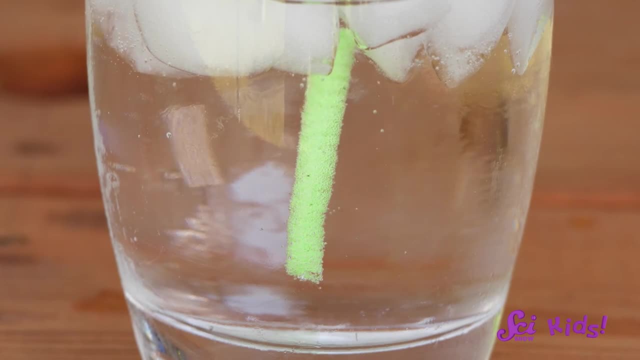 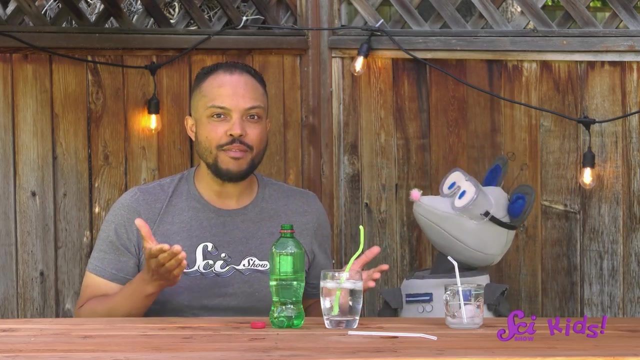 Oh look, there are a ton of bubbles on the chenille stick- way more than the straw. It really helped the bubbles come out more quickly and I know a way we can make it even faster. But this is gonna get messy, so it's a good thing we're outside. 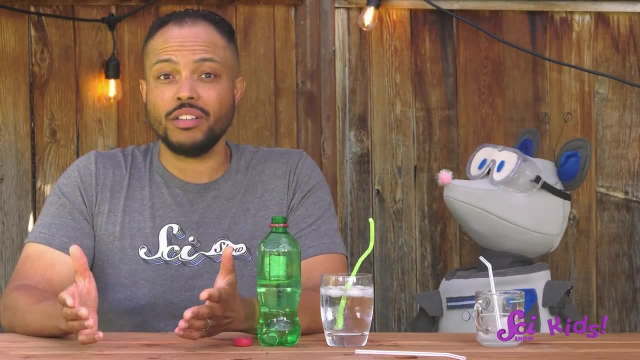 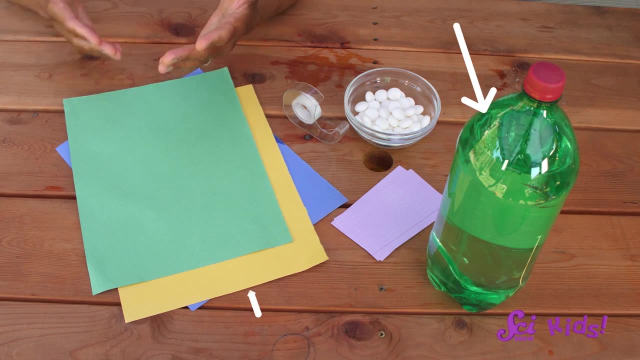 If you wanna try this at home, you're gonna need some help from an adult and you should definitely wear safety glasses or goggles. We're gonna use a bottle of diet soda, some construction paper, a card, some tape and a pack of candies called Mentos. 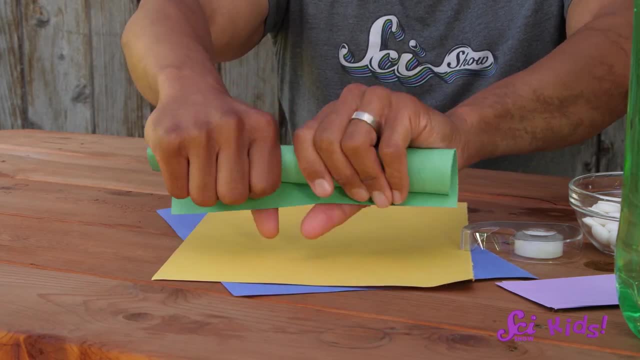 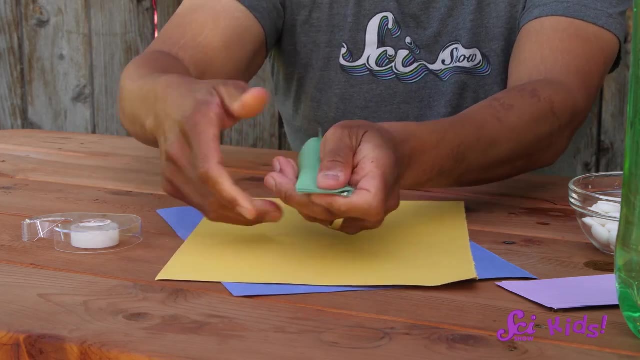 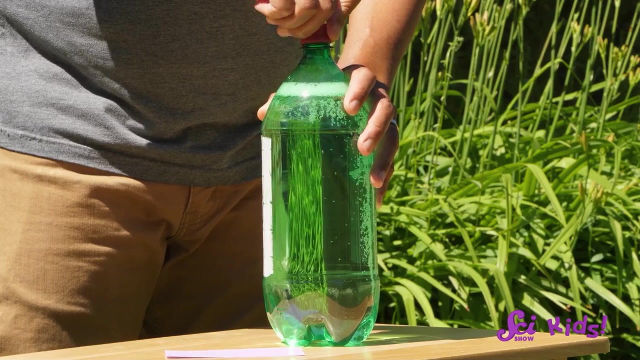 First we need to make a tube from the construction paper and tape it closed. Next we'll close off the end of the tube and put all of the candies into it. We'll put our bottle of diet soda on a nice flat spot and open it very carefully and put the lid aside. 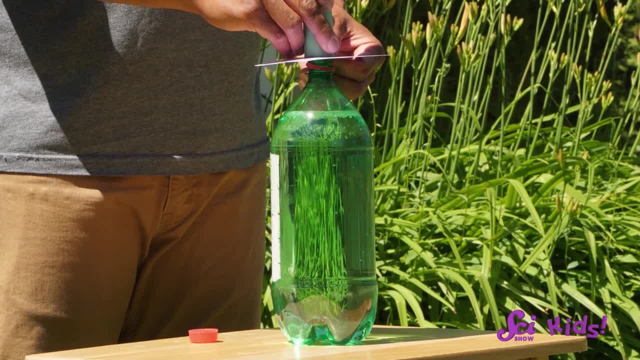 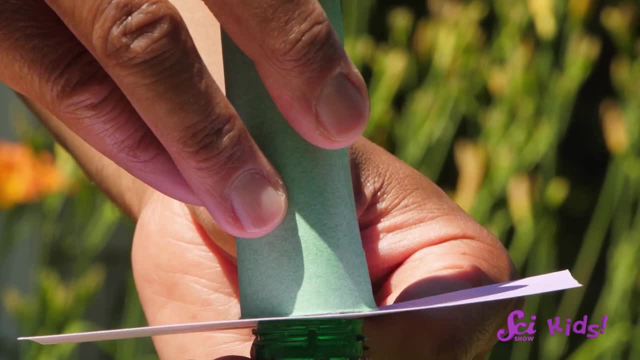 Now we'll put a card over the top of the bottle and put the open end of the tube on the card. We want to line up the opening of the tube with the opening of the bottle. I think we're ready. Let's count to three and then we'll pull the card out. 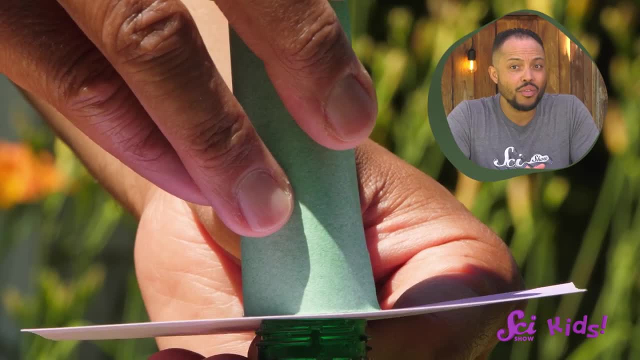 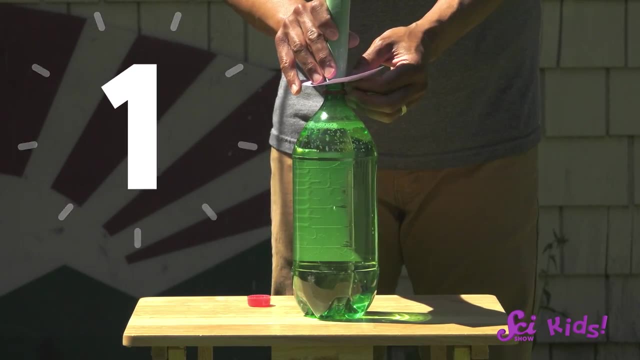 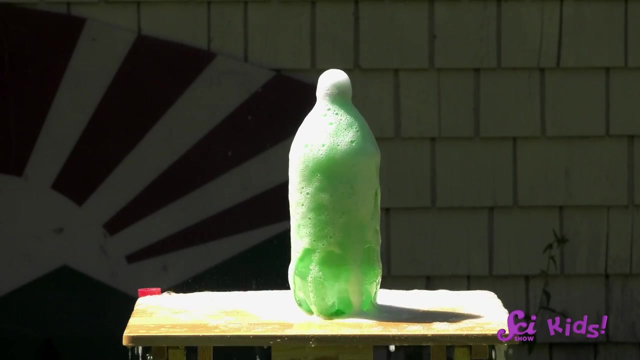 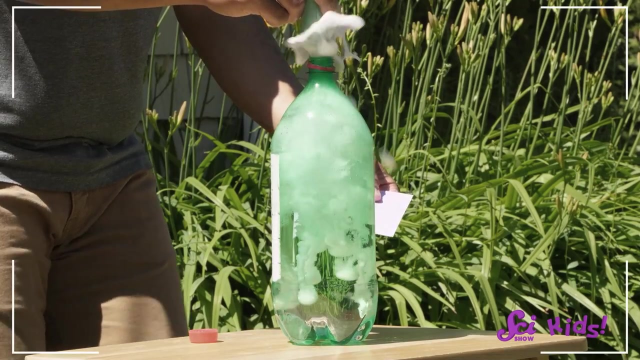 from beneath the tube, so all of the candies fall into the soda bottle at once. Count down with me: Three, two, one go. Wow, that was amazing. The soda squirted out of the top of the bottle and went everywhere. 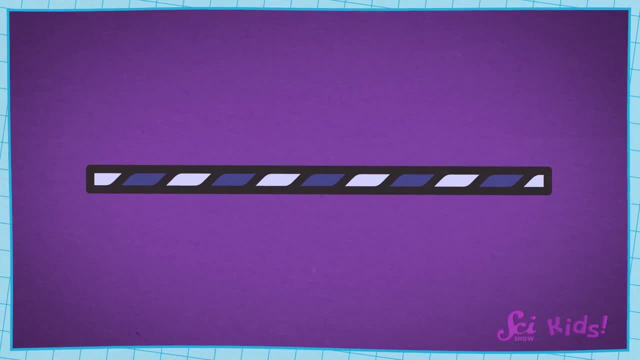 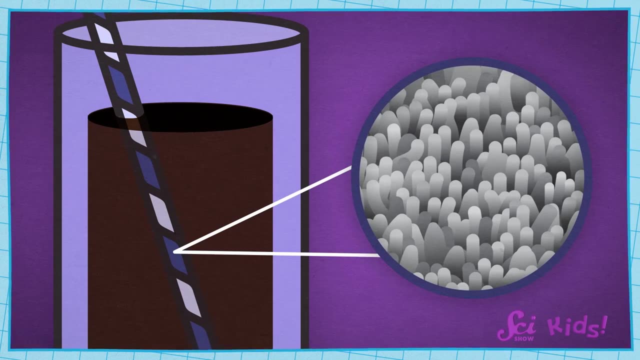 Let's go back to the straw and talk about why, Even though the straw looks and feels smooth, it's really not. If we could look really closely, we could see that the straw has all kinds of bumps on it. The bubbles can stick to these bumps and grow bigger.